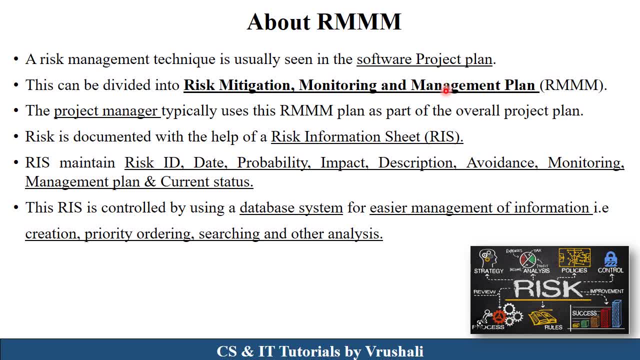 project and management means if risk will be occur, then manage those risk, So this is called as RMM plan. Now this RMM plan documented into the risk information sheet document, which is also called as RIS document. This document stored all the information related to the 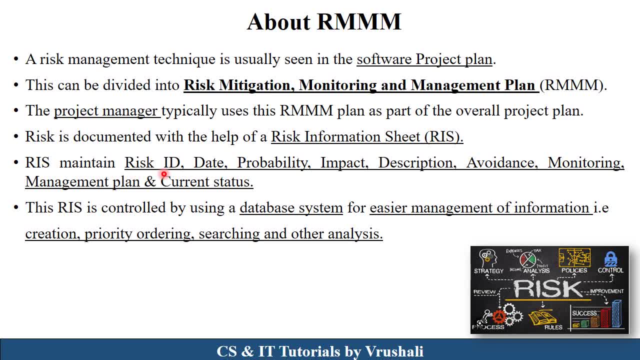 risk in tabular format. They mention risk id, the date where risk have generate, probability of risk, impact of that risk, description about risk, then avoidance, monitoring and management plan and current status of risk. This all information have stored into the risk information sheet. 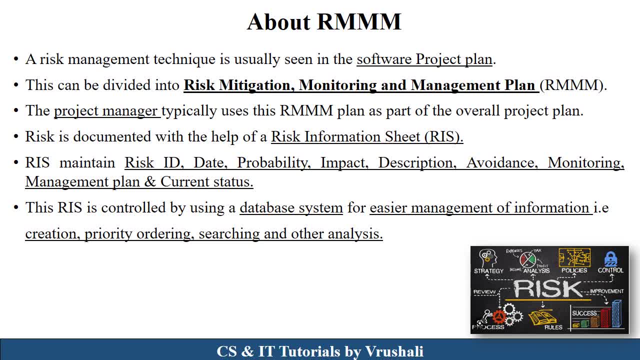 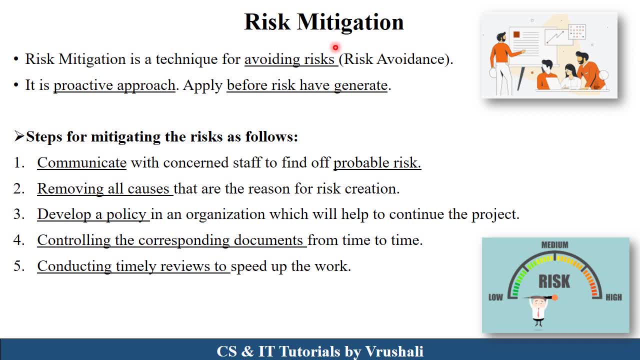 in particular database. Now let understand RMM plan in detail. Now the first thing is risk mitigation. Here project manager identify which type of risk will be generate in particular project in future and how to avoid that risk. This is called as risk mitigation. 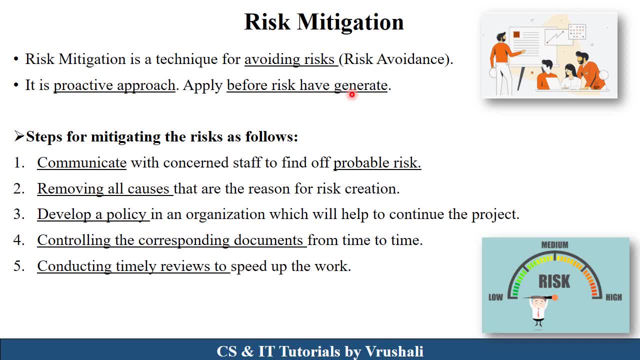 This process apply before risk have generate or early stage of planning phase. That's why this is called as proactive approach. Now these are the steps of risk mitigation process Here. first, project manager communicate with all concern staff and all the stakeholders to find out which type of risk will be generate in particular project, in particular module. 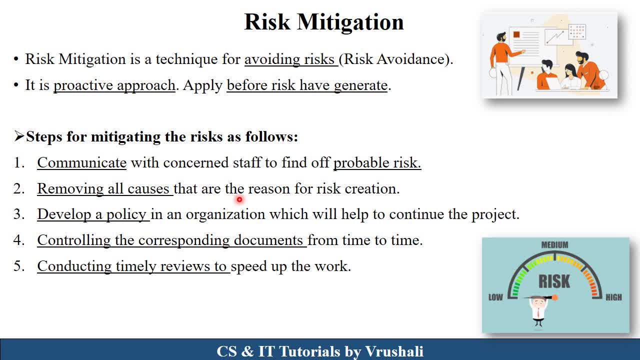 After that they remove all the causes and all the reasons. that's where risk will be generate in particular project. Here project manager develop different policy for an organization or particular software team. They mention some working time of employee, The salary of particular employee, schedule of complete project and they divide the work. 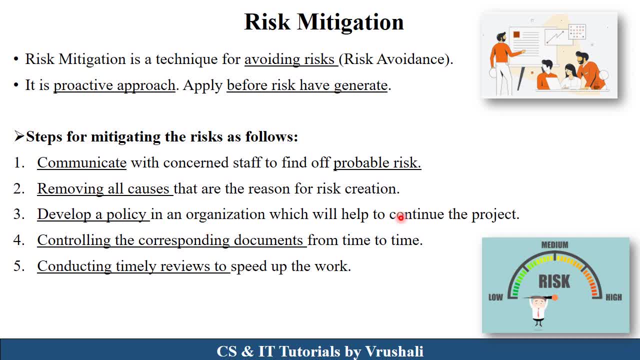 to each and every employee. That's why your project will be going on in accurate manner or in smooth manner. After that, project manager control all the corresponding documents time to time. They check risk information sheet time to time that status of each and every risk. 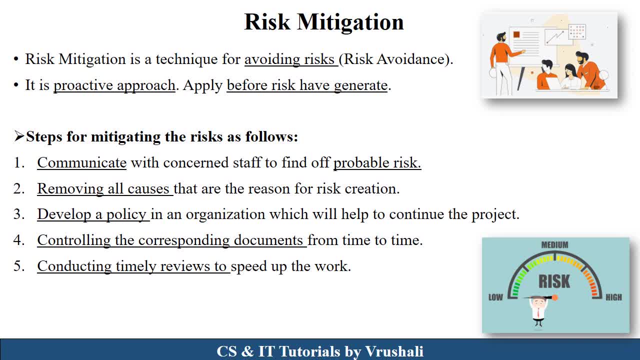 They also conduct timely review or feedback of each and every action. They also conduct timely review or feedback of each and every action. They also conduct timely review or feedback of each and every action. 120. Let's take a look a little bit of what it means for telling you this risk environment. 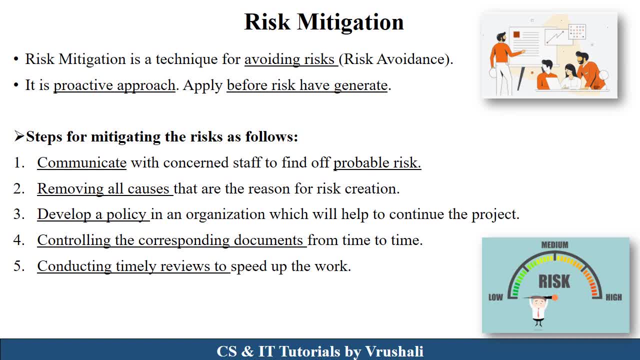 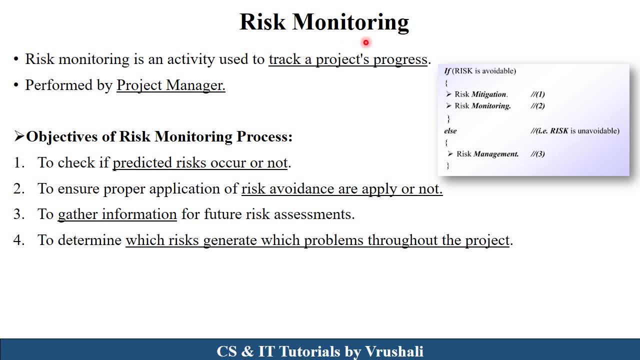 beneficiaries, not19 squares of 154.. clicks movements on pages. the first following candidates: criteria for which category I review tables. Please compare with your project manager name which type of activity that it was: software development life cycle. This is called as risk mitigation, to identify risk will be generate in particular project. 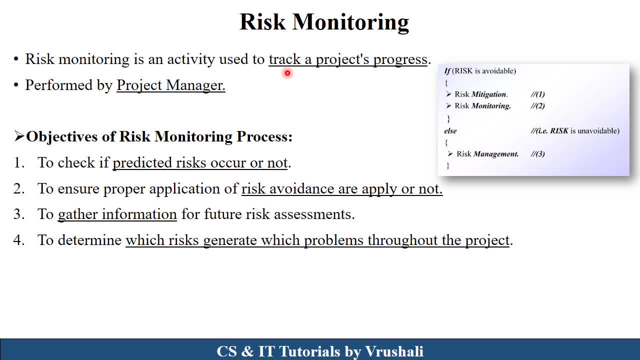 and avoid that risk. 20. Now, after that, the next ben is a risk monitoring. Basically, risk monitoring means your project manager track progress of your complete project. They track which type of activity or which type of software development life cycle will be performed. 23, suggestion 0: COOL SET MARKET RENTり. today you are bracing this particular project. 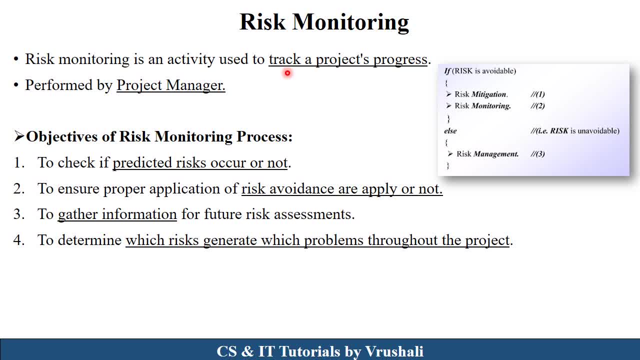 project you would like to interesting about what's going to be carried through, what's going to take. they monitor complete progress of your project. the objective of risk monitoring is here: whatever the risk predicted in risk mitigation process, here project manager check that if predicted risk occur or not. they also check that risk avoidance technique are properly apply or not. 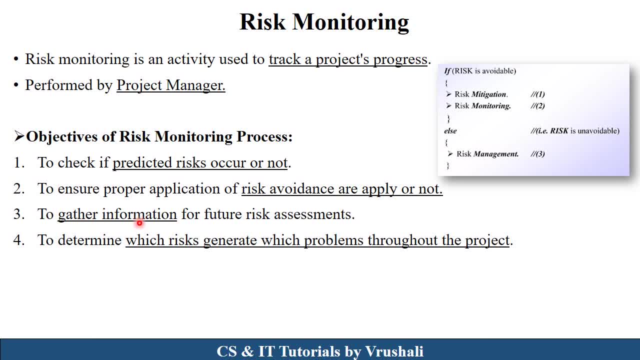 risk monitoring also gather all the information for future risk assessment and here project manager also determine which type of risk will be generate in particular project and after risk generate, which type of impact or which type of problem will be occur in particular project. so this is called as risk monitoring. see here if a particular risk or particular problem in your 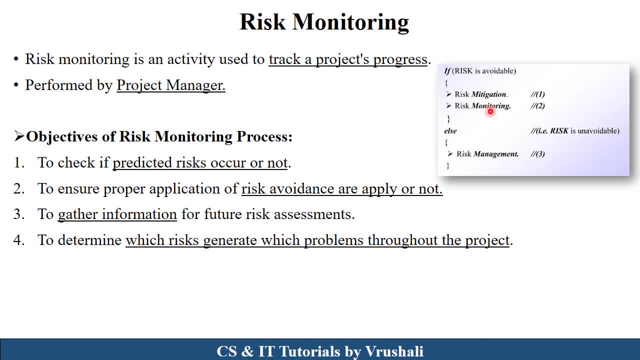 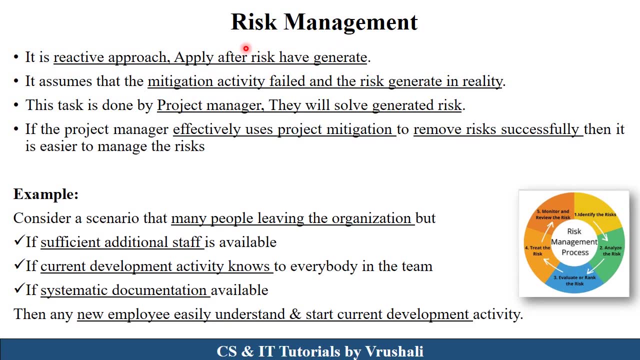 project is avoidable, then risk mitigation and risk monitoring process is performed, but still risk will be generate in future. then risk management technique is performed, so this is called as risk monitoring. now the next thing is risk management. so basically, risk management is performed after risk have generate in particular project. that's why this is called. 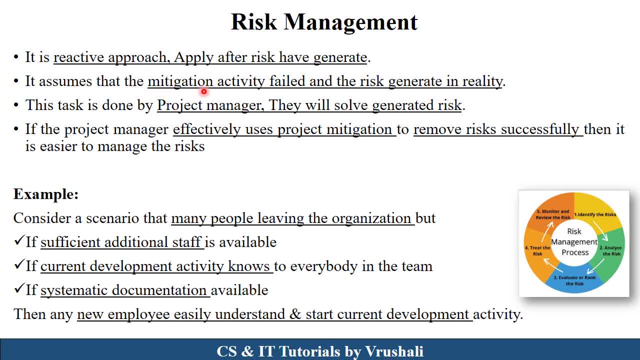 as reactive approach when risk mitigation activity is fail. means project manager first identify which type of risk will be generate and apply some avoidance technique. but this particular activity and automobile and risk generate in reality in your project. so project manager try to solved this generated risk as per some avoidance technique. now see here in this example: suppose consider a 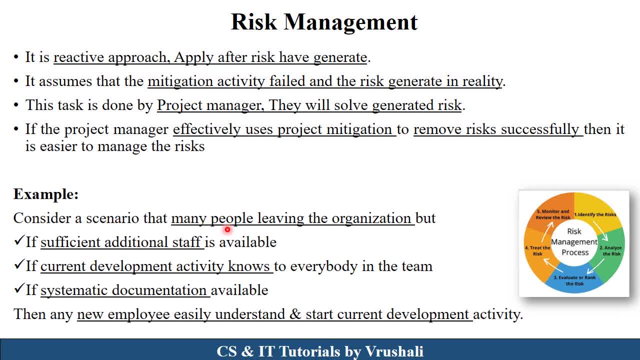 scenario there are many people who work on same project and leaving the organization at the same time. so at that time project manager check that if sufficient additional staff is available or not, or if current development activity or current project is facing such risks, then project manager is notes to all the additional staff, team member or systematic documentation. 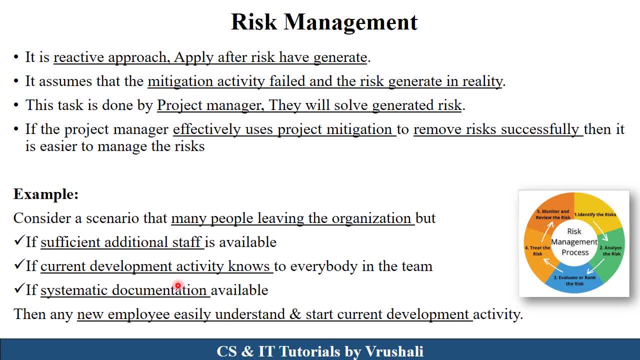 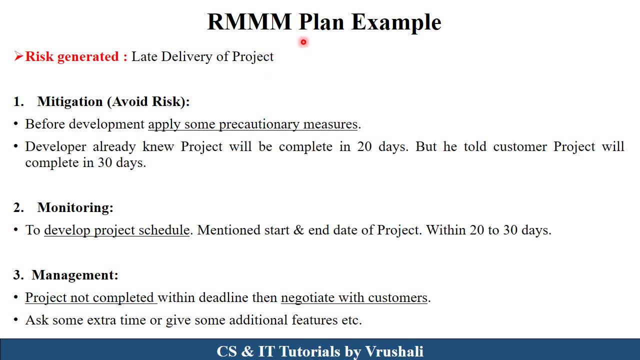 is there. if all these avoidance technique are there, then new employee easily understand and start current development activity. so this is called as risk management process. now see here, this is just an example of RMM plan. you can mention this example as per your exam point of view, suppose in your 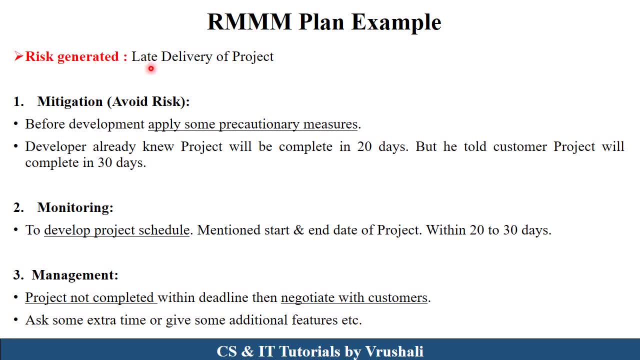 project risk generated and the risk is: late delivery of project means project manager did not complete the particular project within the schedule or within a deadline. right now, what is RMM plan? the first one is risk mitigation. risk mitigation means avoid risk. your project manager identify that late delivery of 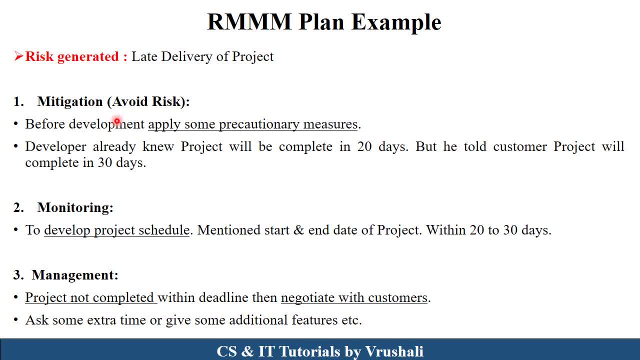 project. this risk will be generate in particular project. so they apply some avoidance technique, they apply some precautionary measures. you can see here: this is the RMM plan. this is the RMM plan. this is the risk management process. how see here? so here: developer already knew that project will. 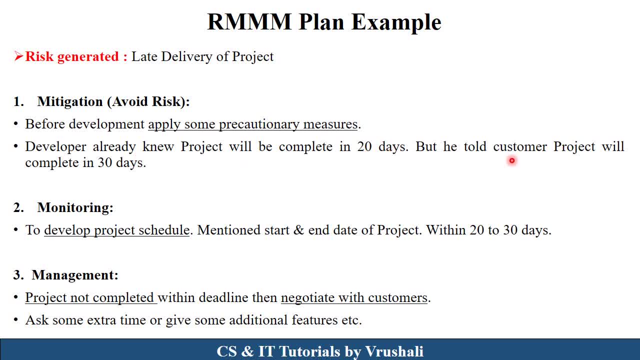 be complete in 20 days, but still developer told customer about project will complete in 30 days means developer take 10 days extra for completing a particular project. so this is called as precautionary measure and this is called as avoidance technique. now the next one is a monitoring. so here, project manager. 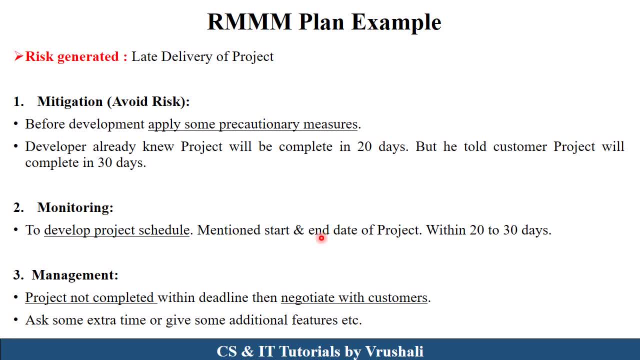 develop a particular project schedule, mention start and end date of project, complete project or each and every activities perform in particular project. this is called as risk monitoring and at the end there is a risk management means. after apply mitigation and monitoring, still risk have generate. your project is not completed. 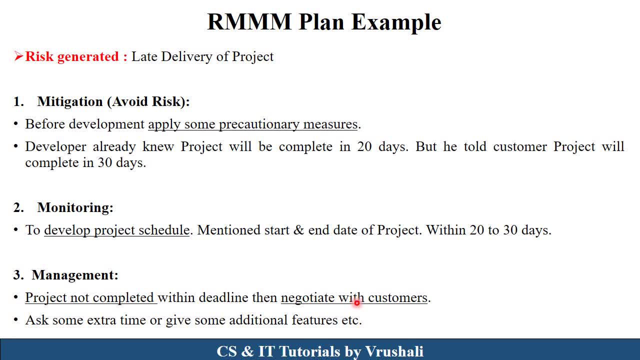 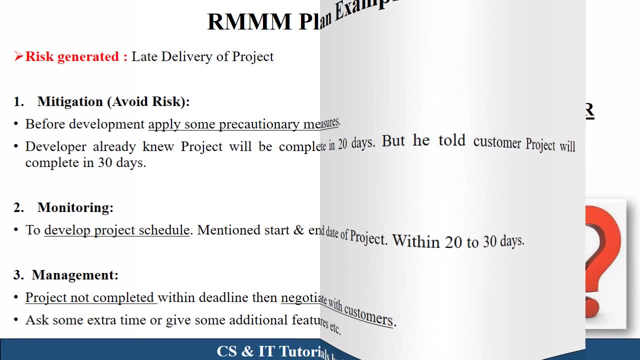 within a deadline. so at that time project manager negotiate with the customer. they discuss with customer, ask some extra time. also, developer give some additional features to the customer. so this is called as RMM plan, the risk management. so this is a example of RMM plan. now, as per your exam point of: